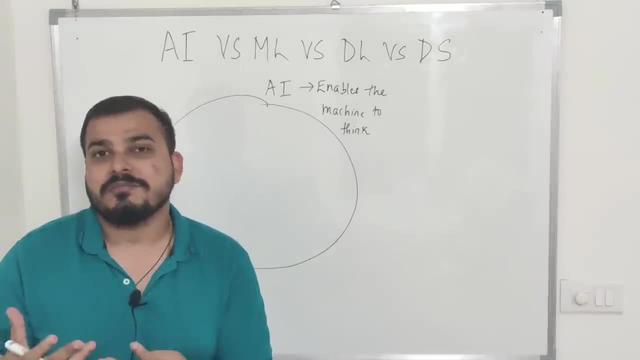 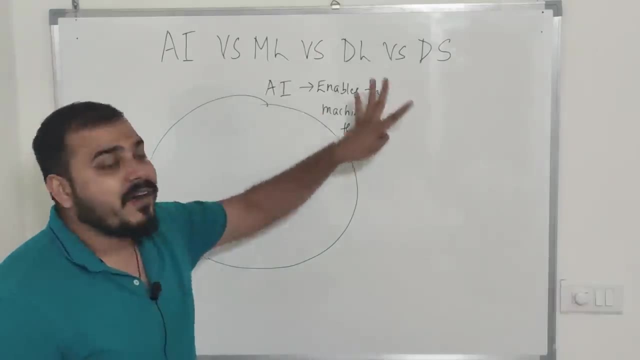 a self-driving car, that is an ai application. an application or app which actually uses machine learning and deep learning within them is basically an ai application. it does some kind of task. so, finally, this is my final goal: i have to reach over here and create an ai app. okay, now when? 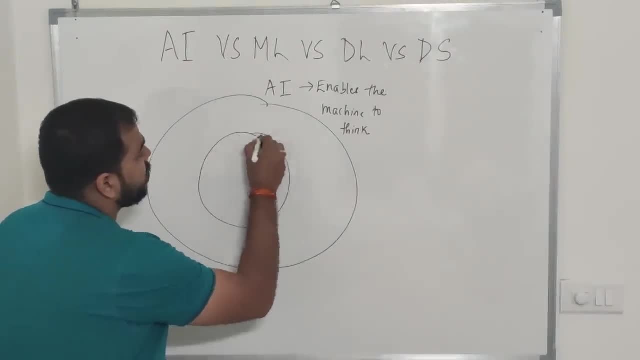 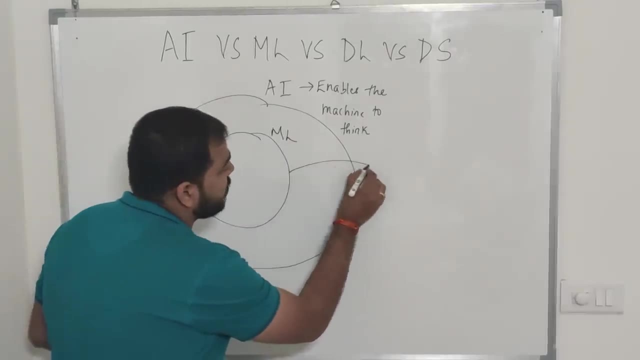 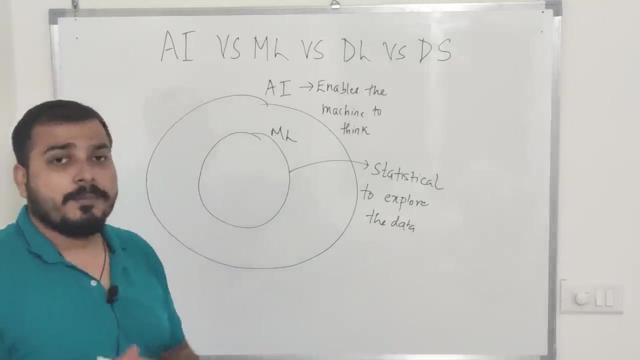 i talk about machine learning. machine learning is a subset of ai, learning is a subset of AI. and what does machine learning help us to do? it provides us statistical tools. statistical tools to explore the data, to explore the data, simple definition guys. it provides us some statistical tools to 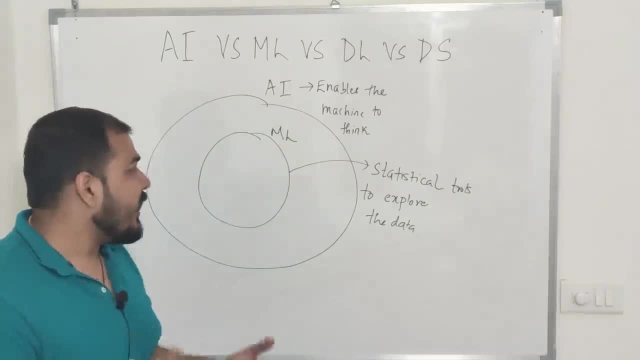 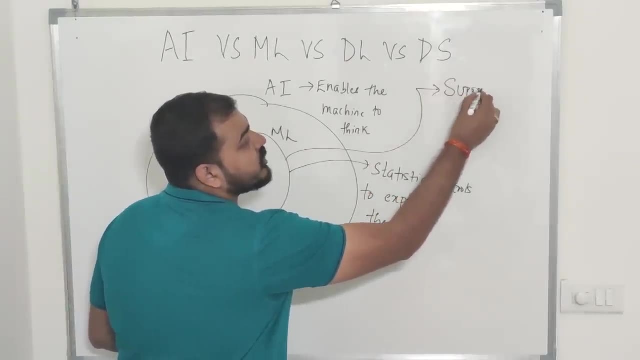 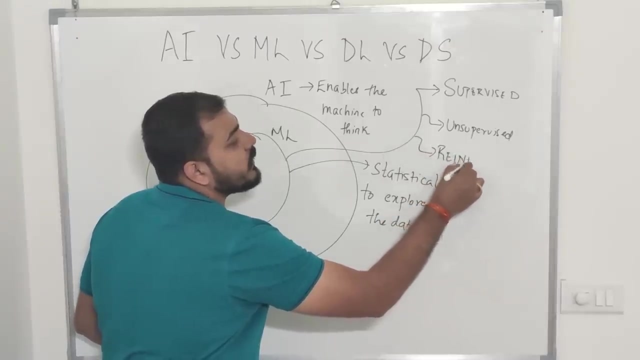 explore and understand about that particular data. now when I talk about machine learning, in machine learning you have three different approaches. one is supervised machine learning. I'll also discuss about what exactly supervised, okay. so second technique is something called as unsupervised machine learning. the third technique is something called as reinforcement- reinforcement learning. 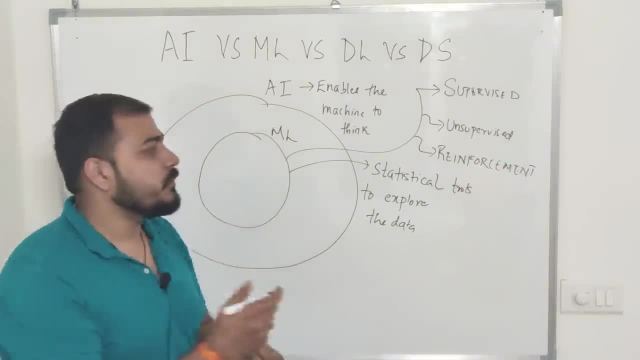 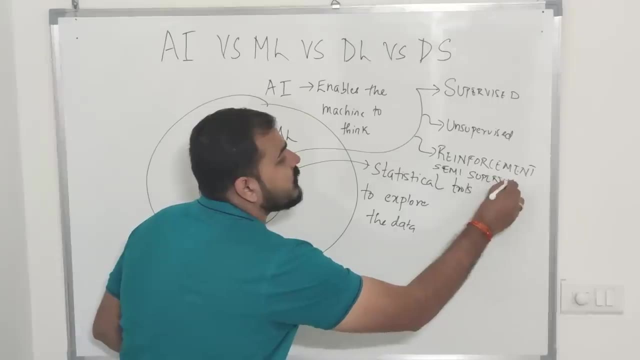 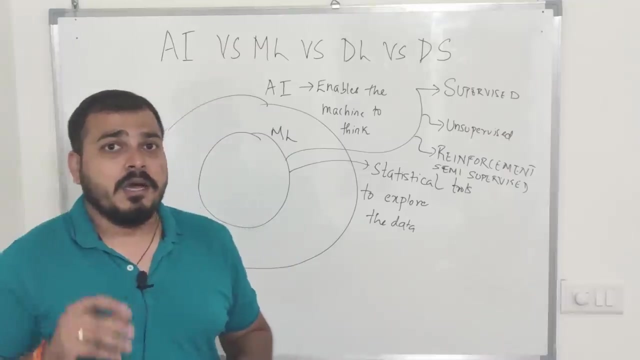 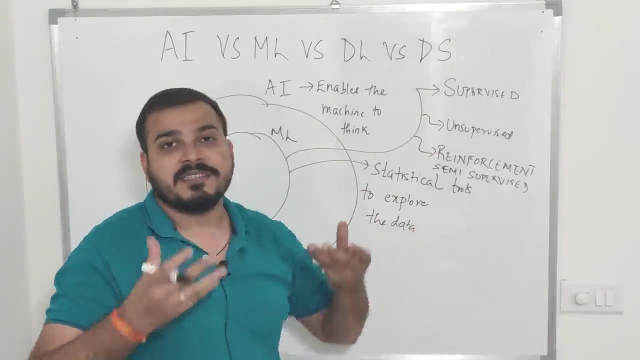 or this is also called as semi supervised machine learning. okay, I can write it as semi supervised. so this techniques of machine learning is basically ranging in this. let me give you a very good example of supervised. so in case of supervised will be having some label data, you know, some past data and with the help of this, 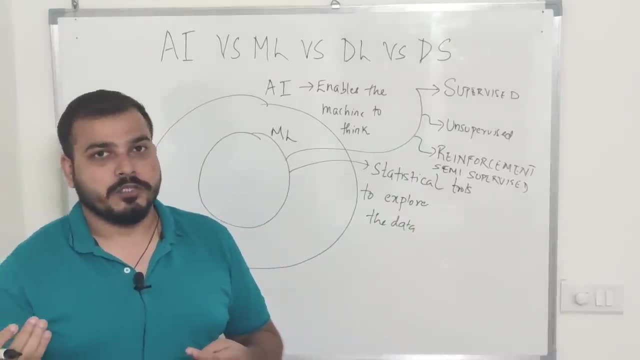 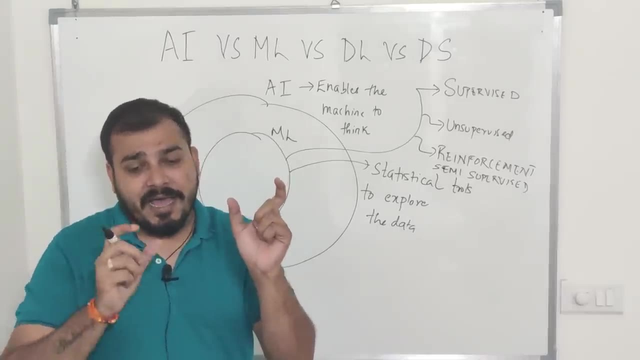 kind of data will be actually able to do the prediction for the future. let me just take a very good example, suppose, based on I have two features in my data set like age. I have. I have not age. let me just consider that I have height and weight as my two features and 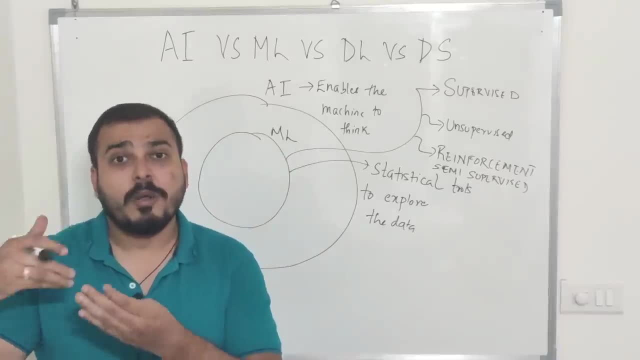 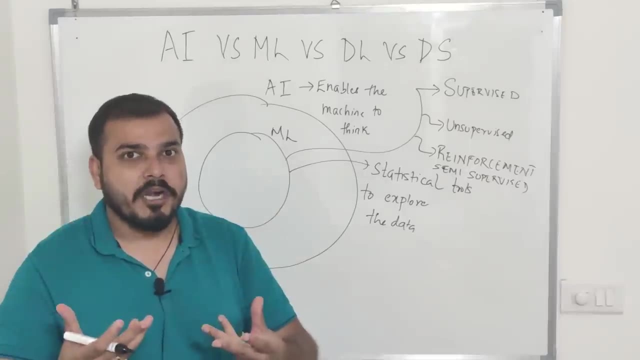 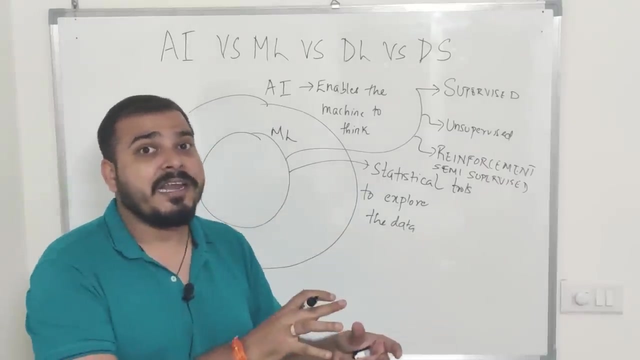 I want to classify whether that person will is belonging to an obese category or whether it belongs to the fit category. right, so this kind of data initially, whenever I'm making my model. at that time I'll have this data in hand previously only, and what I'll do? I'll create a model, train on that data and 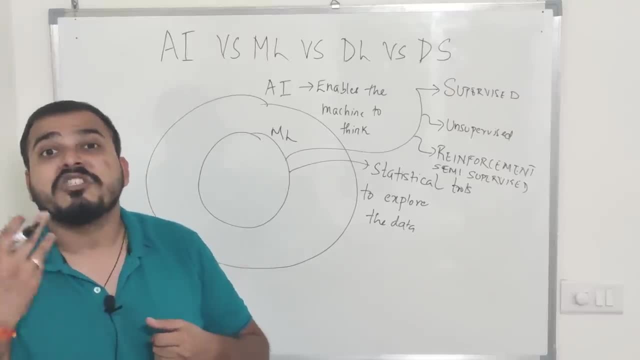 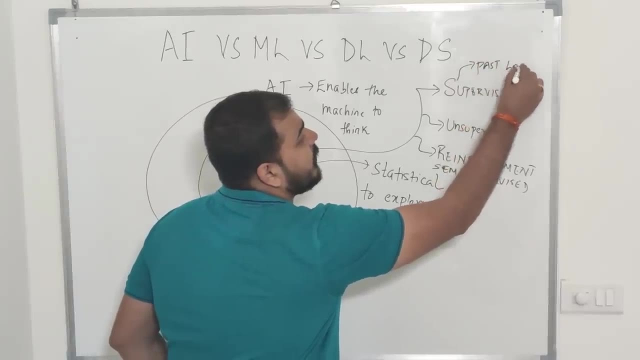 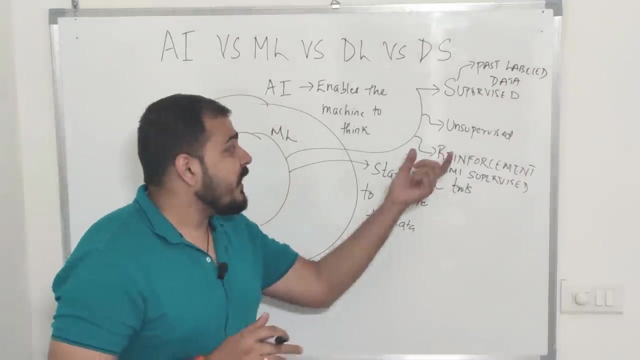 with the help of those kind of data, I'll be actually creating a supervised machine learning model. that basically means so, in case of supervised, we have past data, past labeled data. okay, we know what will be the output of this particular data. now, in the second category, when I talk about unsupervised- 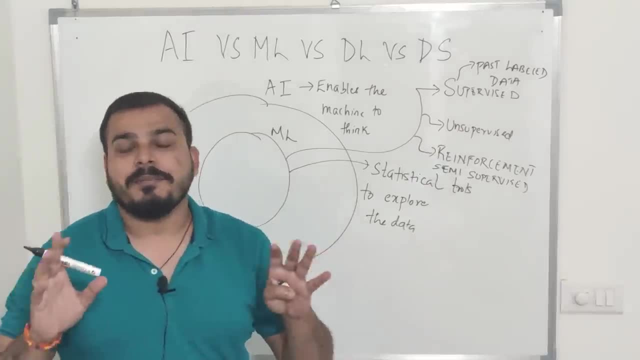 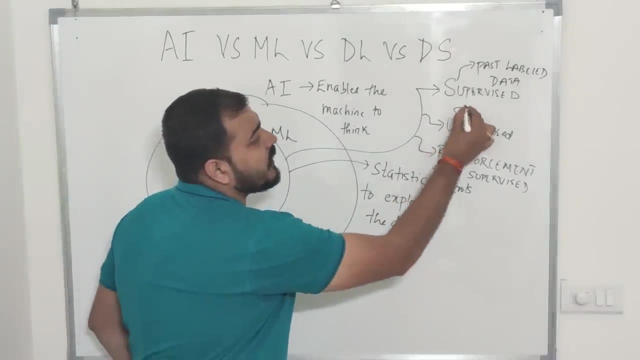 machine learning. here I'll not be having any labeled data. that basically means in my data set I will not know what is the output. so in unsupervised machine learning we usually solve clustering kind of problems. clustering, you know they are different, different clustering techniques, like k-means clustering. 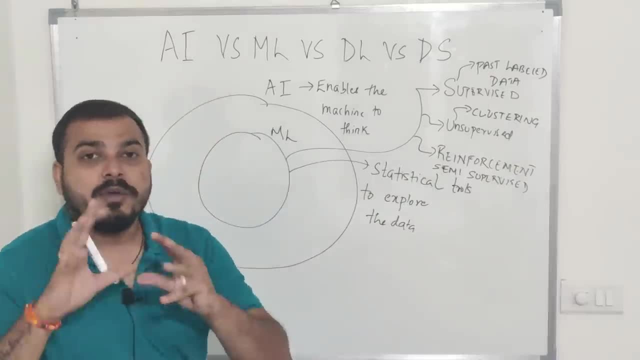 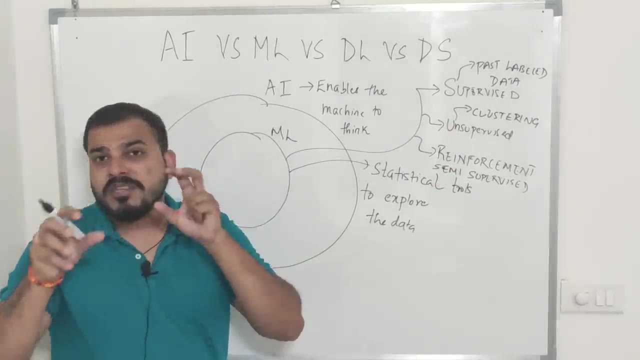 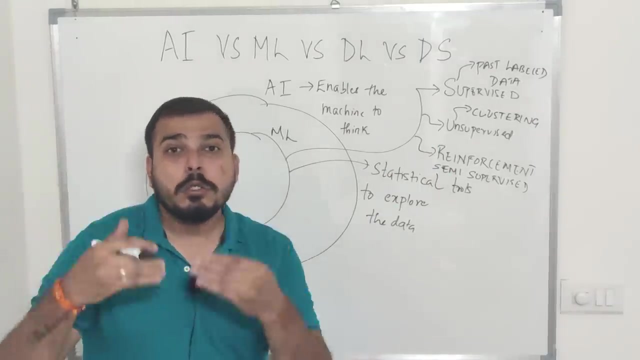 hierarchical mean clustering. so in unsupervised machine learning we will actually be solving clustering techniques. and when I say clustering, what exactly it does is that, based on the similarity of the data, it will try to group that data together. and there is some mathematical concepts like Euclidean. 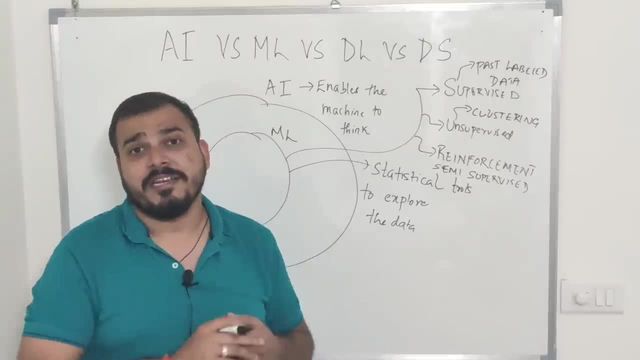 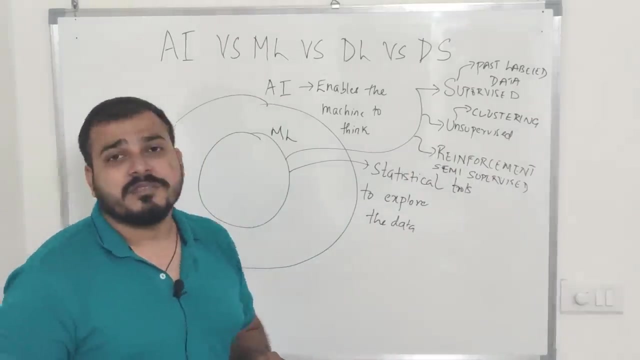 distance actually used inside that with apart with some other techniques also. so most probably here are two different algorithms or three different algorithms. one is k-means clustering and the other one is clustering. k-means clustering, hierarchical mean clustering, DB scan clustering. these are the three popular clustering algorithms that we basically used in unsupervised. 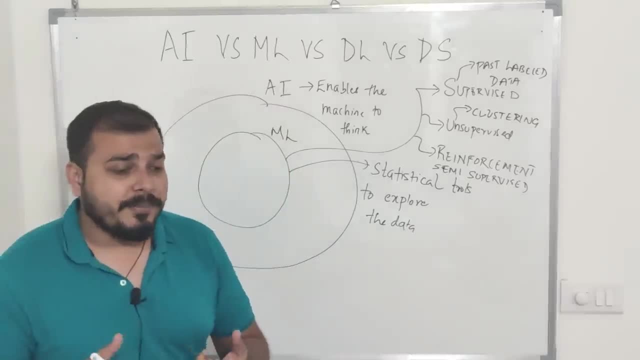 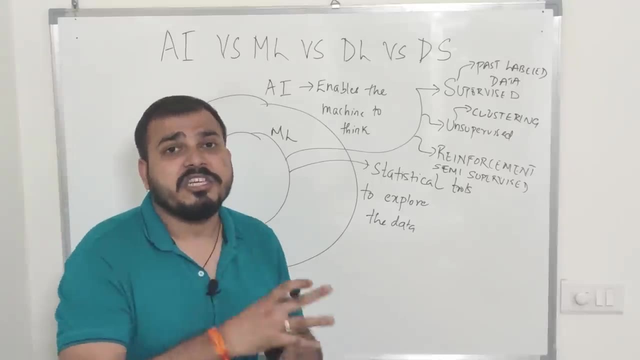 machine learning. now, in case of reinforcement learning, what will happen is that some part of your data will be labeled and later on some part of the data will not be labeled. so the computer or the machine learning model learns slowly by seeing the past data and it will be learning as soon as the new. 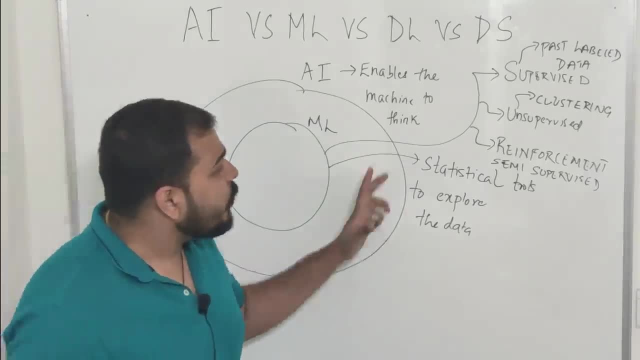 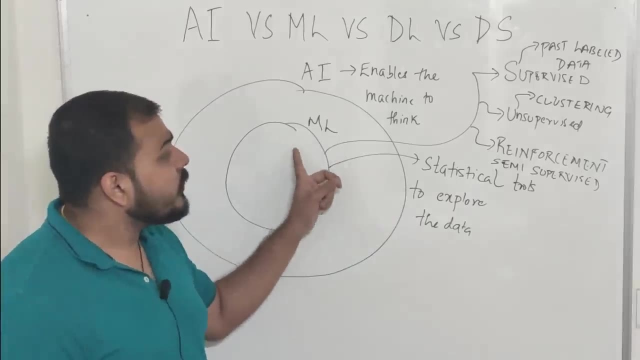 environment. new, new data will be coming up, so I hope you understood this. that is what we are actually learning today doing over here. the most important part is that we need to have data. it also it also provides on statistical tools to analyze, explore and analyze the data. 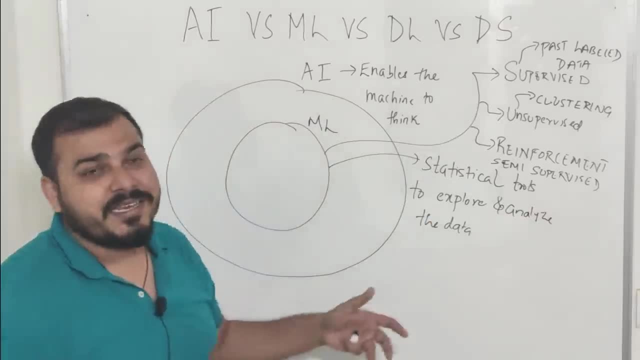 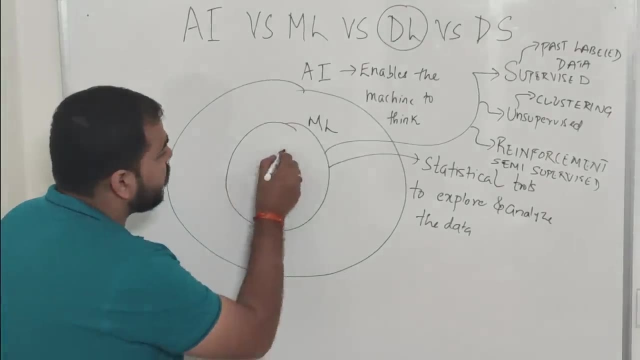 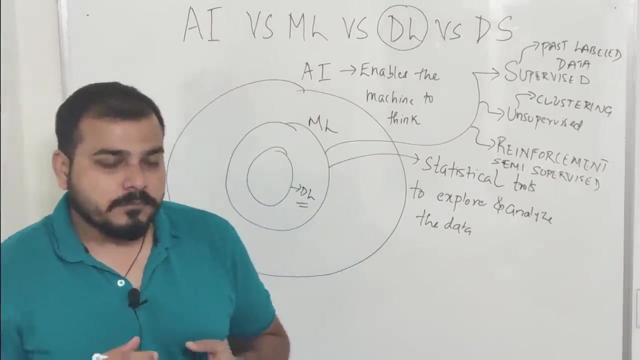 okay, and this is the three different techniques that we basically have in machine learning. the last, the third part, which is my deep learning, is again a subset of machine learning. now, why did deep learning got created, you know? so what scientists thought is that can we make the machine learn? like, how do we? 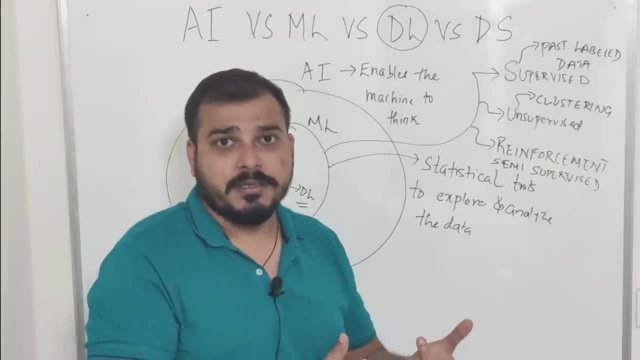 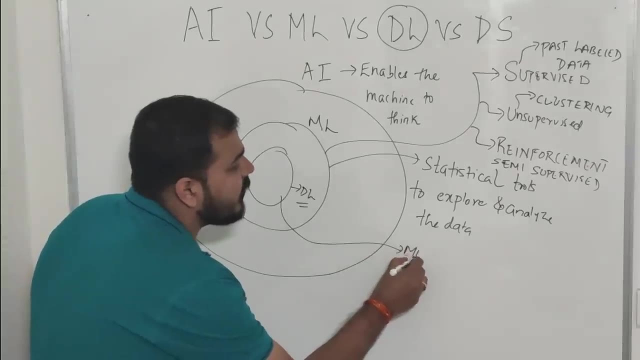 with the help of human brain, actually try to learn things. you know, that was the main idea behind deep learning. so over here in deep learning, you create architecture which is called as multi neural network architecture, multi neural network architecture. so at the end of the day, we are basically using multi. 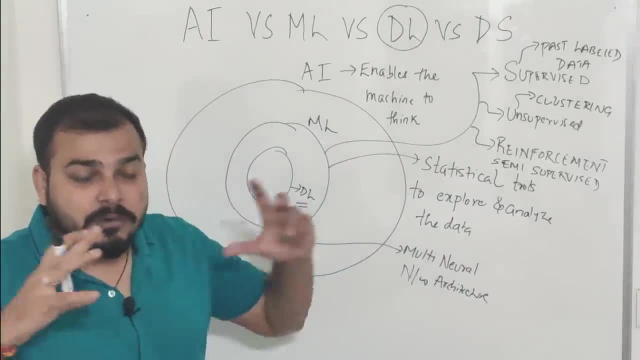 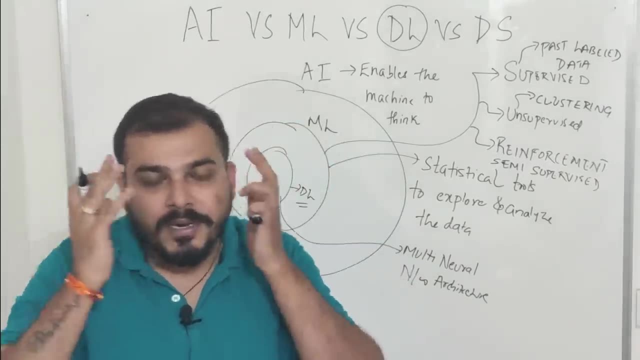 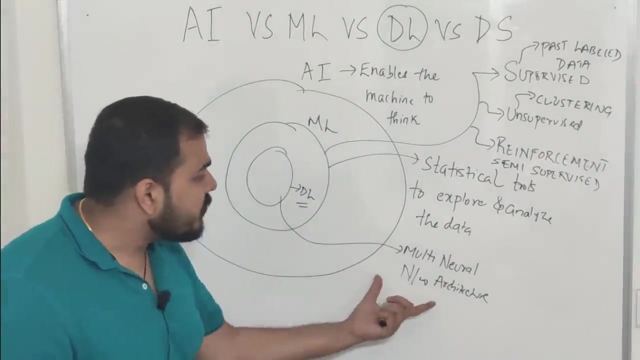 neural network architecture and we are actually creating some deep learning neural networks. the main idea behind deep learning is to to mimic human brain. you know how human actually learns those concepts. similarly, we are creating models over here which is learning those things and the most important thing is multi-neural. 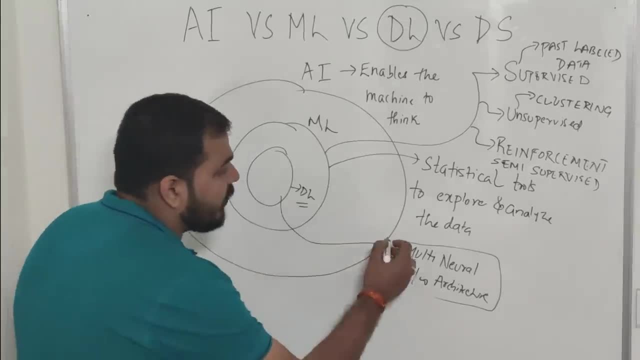 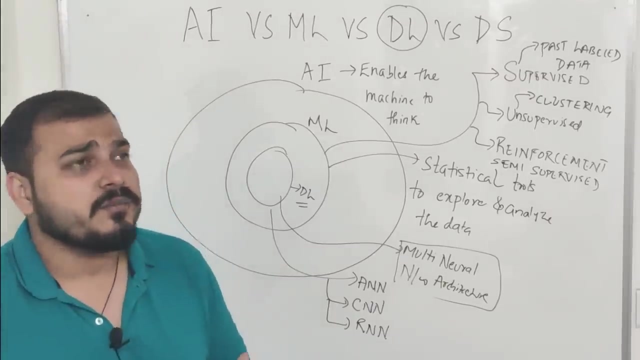 network architecture right, and in deep learning also, you have various techniques. one is ANN, that is artificial neural network, the second one is CNN, that is convolution neural network, and the third one is RNN, which is called as recurrent neural network. most of the problem statements, most of the data which is actually present in the form of numbers, will be solved with the help of 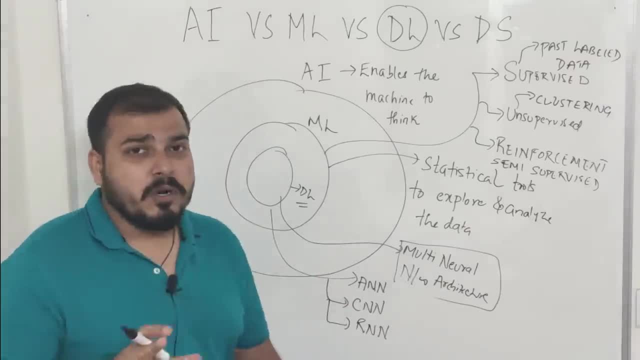 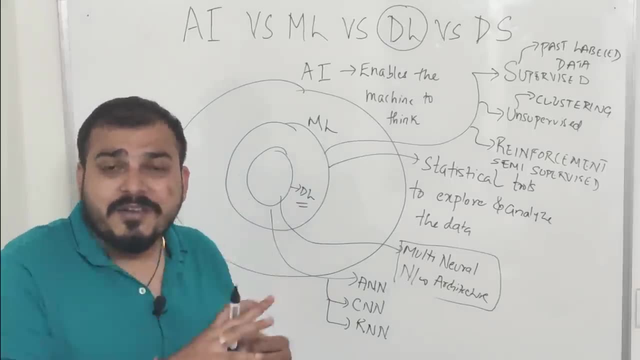 ANN, you know artificial neural network. suppose our input is in the form of images, we will basically use CNN, that is, convolution neural network, and suppose if our input is in the form of time-series kind of data, at that time you will be using recurrent neural network. apart from this, 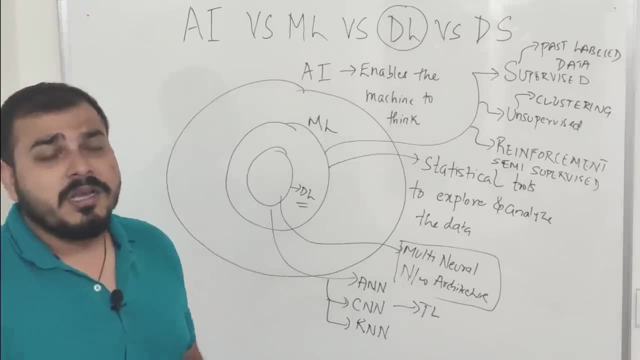 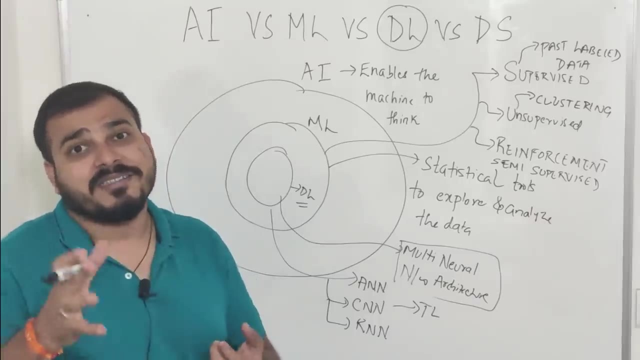 there are also techniques like transfer learning. you know there are some advanced neural networks, extension of the CNN and one CNN. so if i take an example of mask or cnn, right? so these are some advanced neural network architecture which, where the base, is actually a cnn architecture. so you should try to understand this first of all. 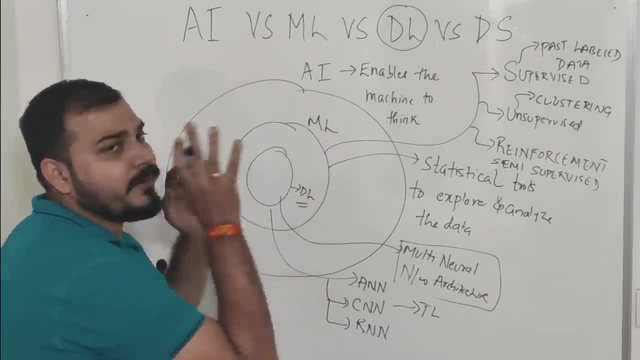 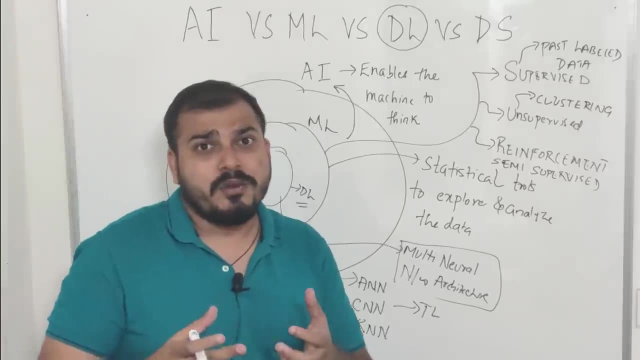 i am actually using this concepts of machine learning and deep learning, and the main goal is to derive an ai application. you know, by using this particular techniques. i want to. i want to create a model which will be: i want to create a self-driving car. so that is self-driving car. 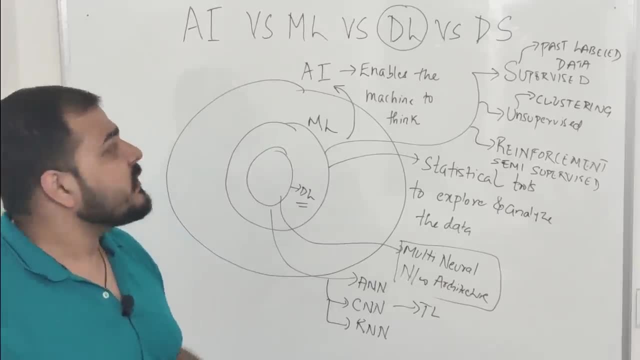 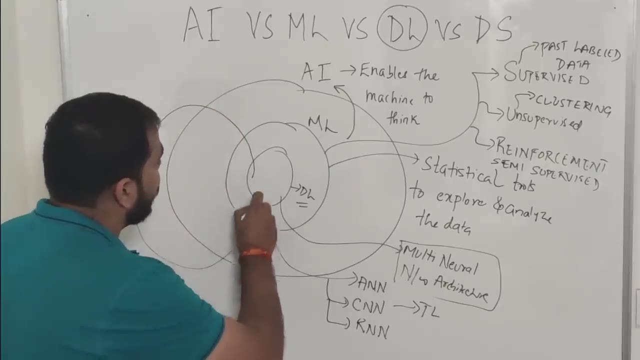 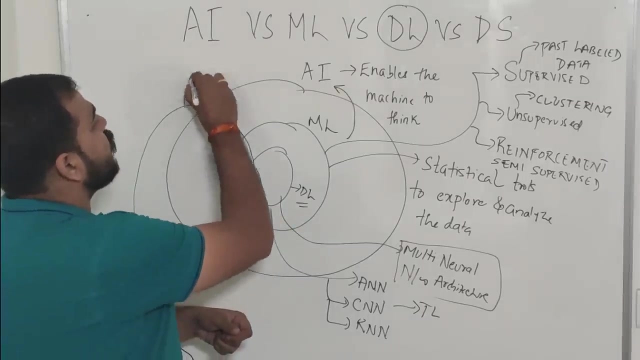 maybe an ai application. okay, now the question arises: where does data science fit into this? right now, data science is a technique which tries to apply all. this particular part means all these techniques. that has basically machine learning, deep learning, and apart from that, it also uses some tools, some some, some some mathematical tools like statistics. you know probability. 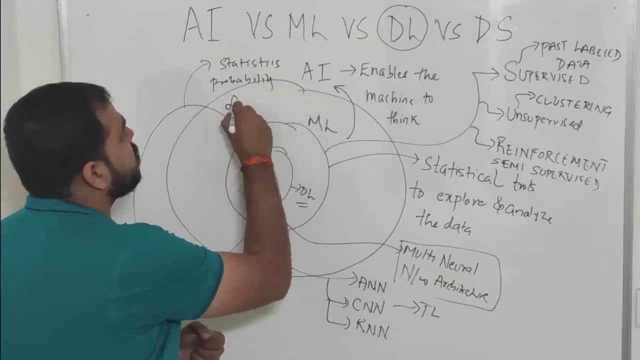 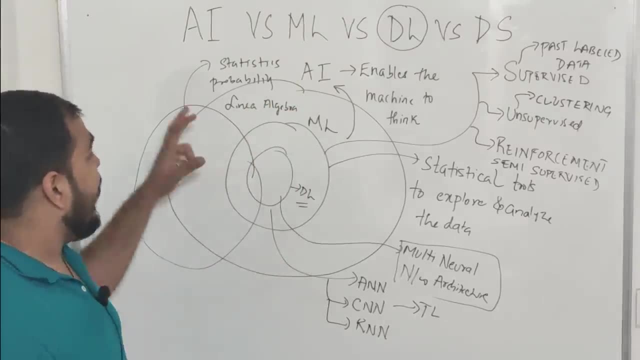 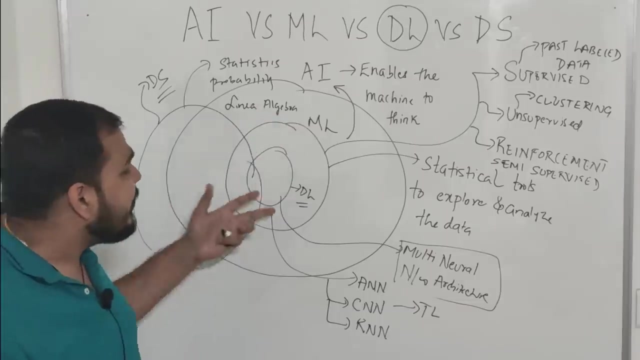 linear algebra, linear algebra, a whole lot of different, different maths like differential calculus and all right, and that is what this is basically my ds. that is data science. so a data scientist will have to work on ml, dl, based on the type of use case, by using some mathematical tools like statistics, probability.